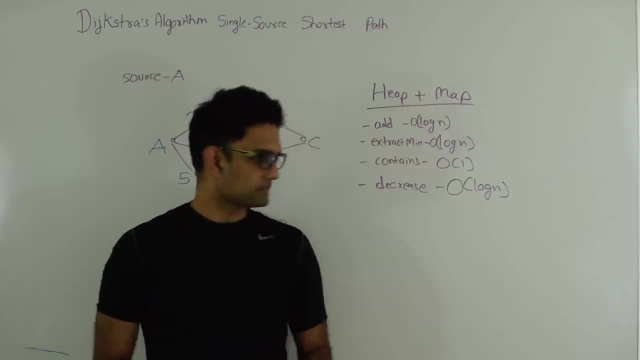 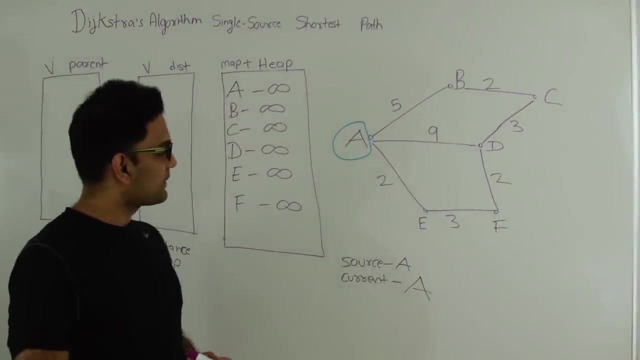 that video first, before watching this algorithm here. So now in the next section, let's see how Dijkstra's algorithm works. So we are going to run Dijkstra's algorithm on this undirected graph here. Here the source vertex is A and we are trying to. 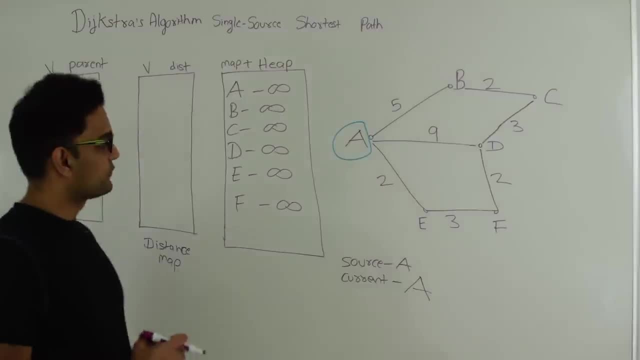 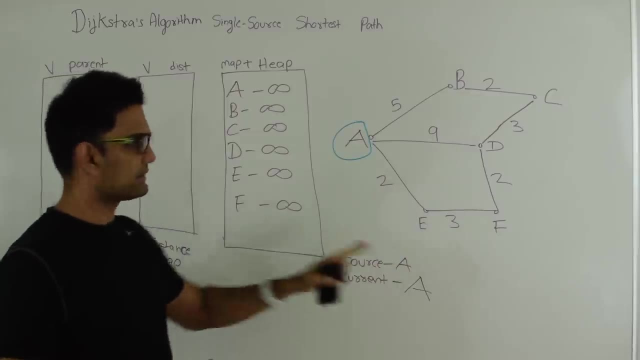 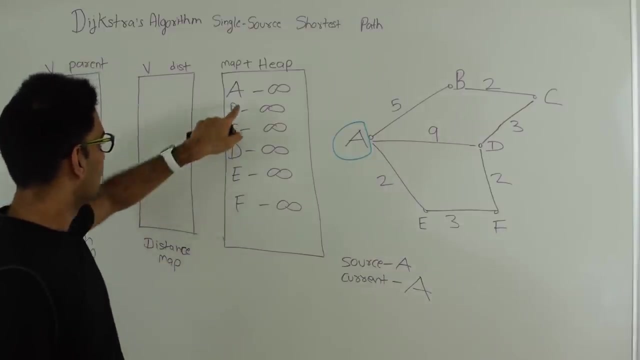 find the shortest distance of every other vertex from A. So the way this algorithm works is: I have this heap plus map data structure and then I'm going to put all the vertices in this data structure with the distance infinity from A, because we don't know how far they are from A at this point of time. Then we're 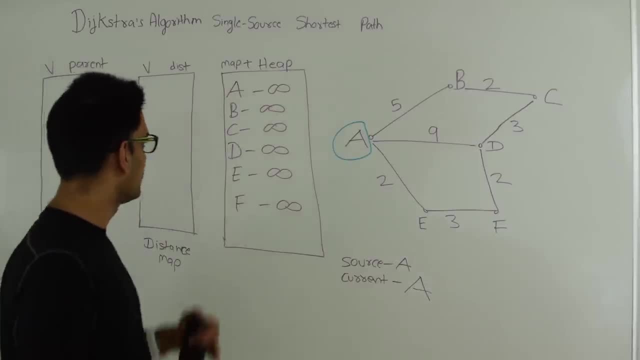 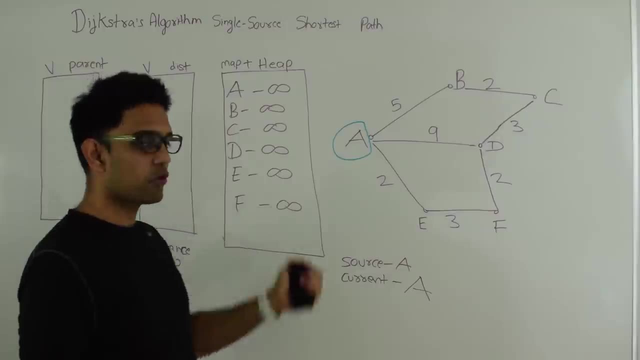 going to set A's distance to zero, because A is a distance zero from itself, and then we're going to do an extract mean here. so basically get A out and then explore all its neighbors and update their distance from A, So we'll get neighbor BDE. 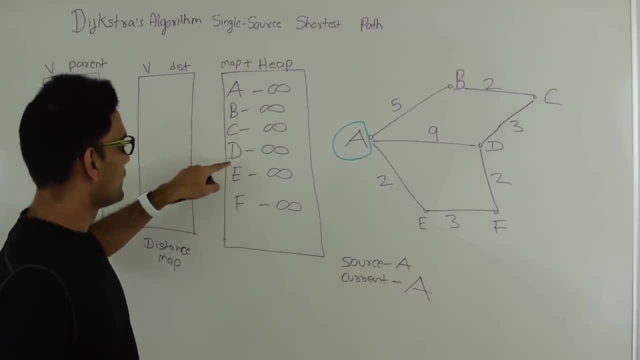 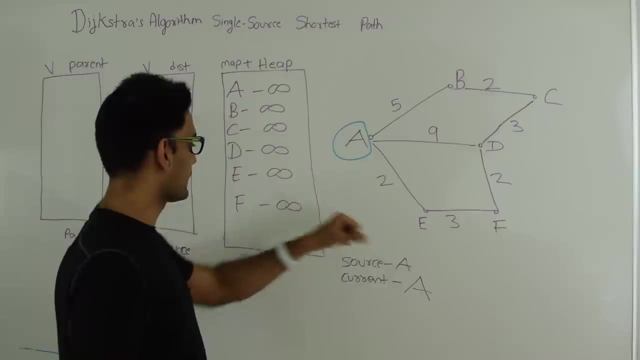 So we'll get neighbor BDE And update their distance so B5, D9 and then E2 from A, and then I'll do another extract mean. so get E out and explore its neighbor. so that's F and the distance of F from A will. 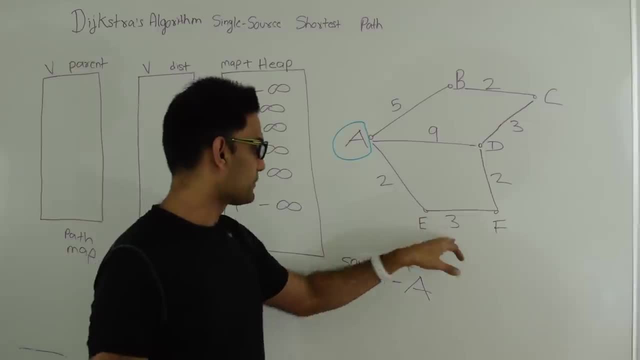 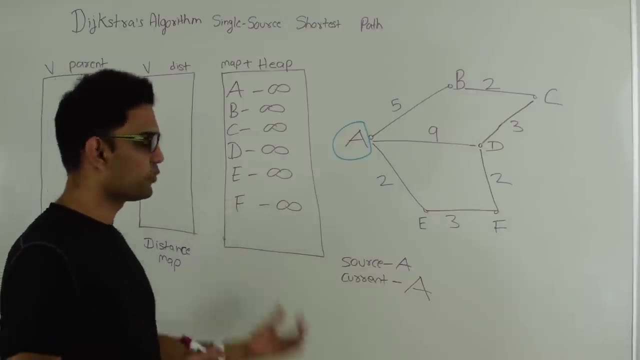 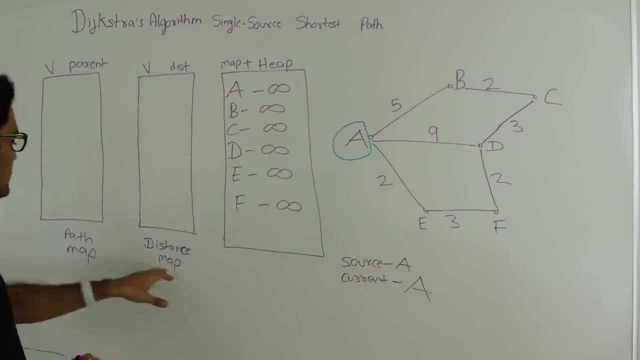 be whatever the distance E is from A and plus this weight here, so that's 5.. So put 5 there in place of F and then keep doing this extract mean until we have a distance, Until we have elements in this data structure here. 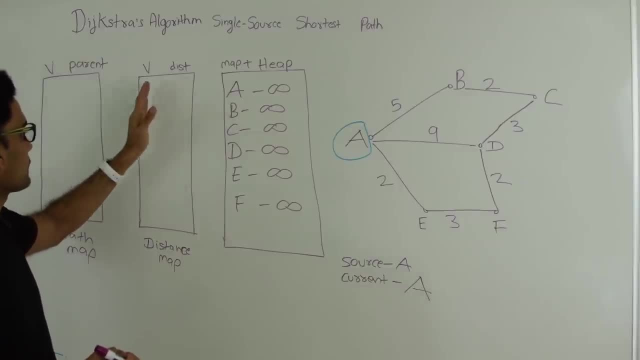 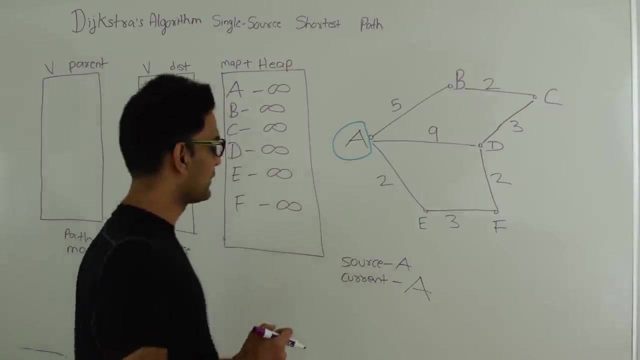 This distance map is going to store the distance of shortest distance of the vertex from A, while this path map is going to help us trace back the path, the shortest path from A to every vertex. So let's do a dry run of this algorithm on this graph here. So, initially, our source vertex. 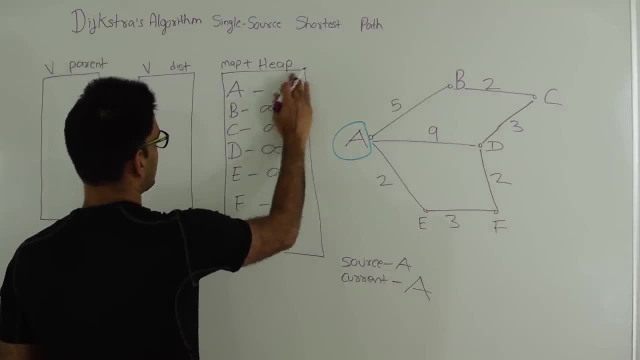 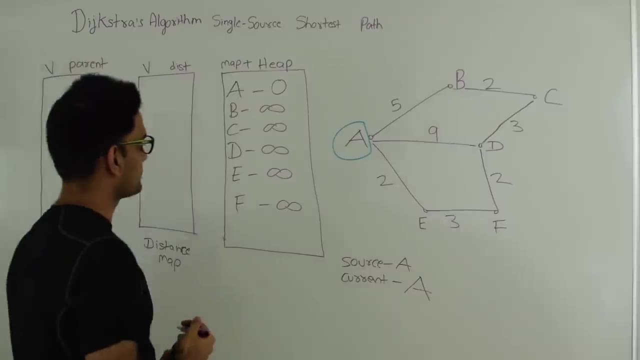 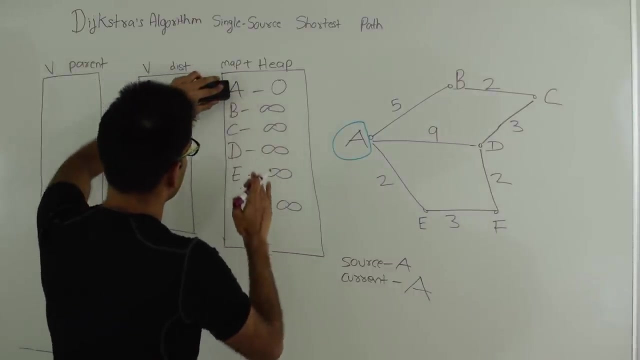 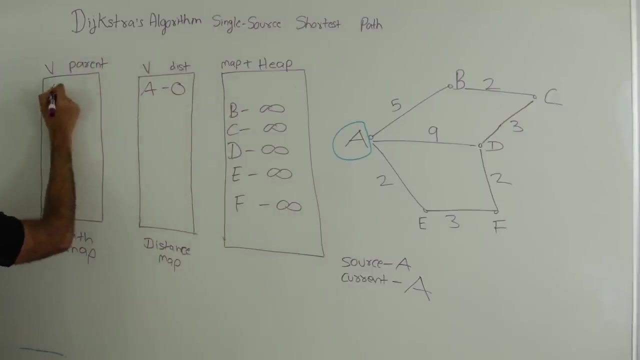 is A. So we put this value as zero. Okay, Then we do an extract mean here and then we make our current as A. So then we're going to explore neighbors of A. So the first neighbor of A is B. So let's first remove A from here and then update A's distance as zero and A's parent. 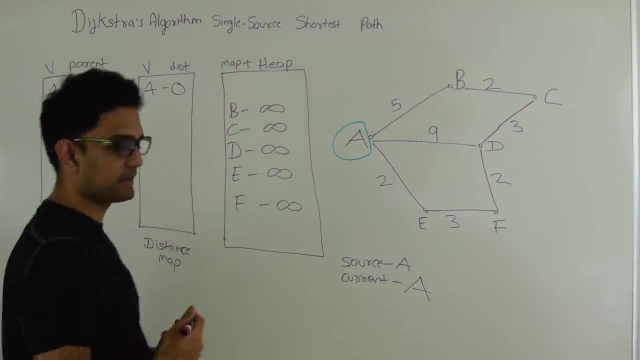 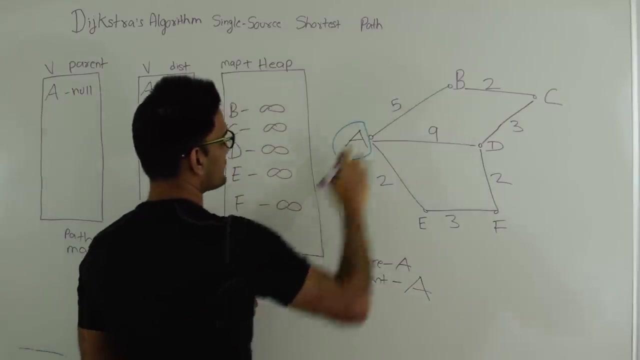 as null, because A is the source vertex. Then you're going to explore neighbors of A. So first neighbor of A is B. So B exists in this map here, yes, And then the distance attached with B is greater than this edge weight here. 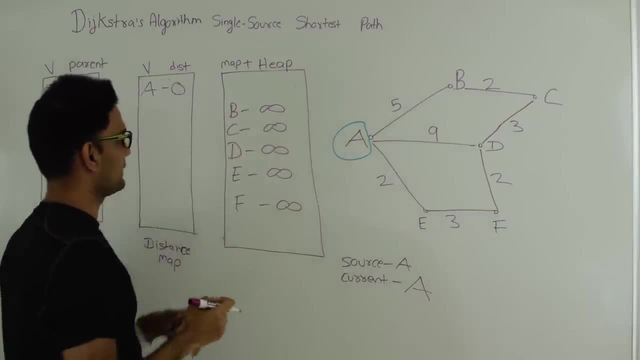 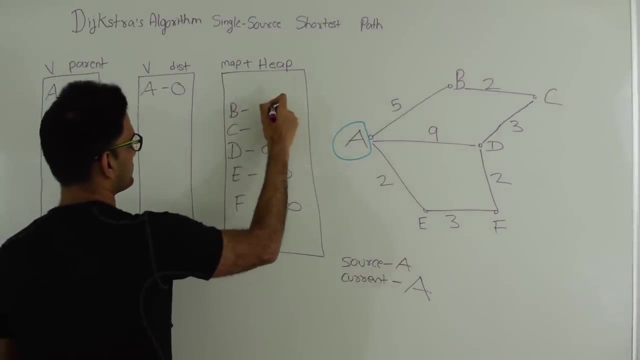 So we'll update this distance to this, Basically saying that we found a path which is shorter than what you know right now. So we'll update this to 5.. Then we're going to explore also, we're going to say that B B's current value is zero. 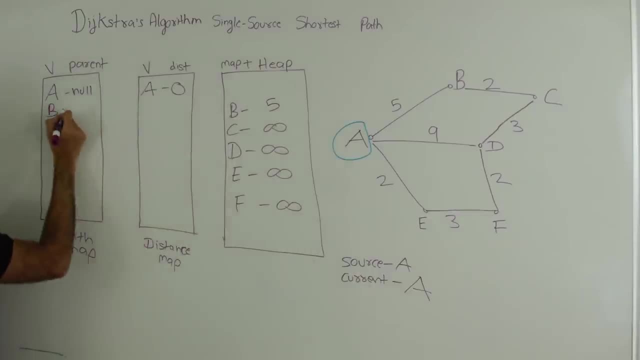 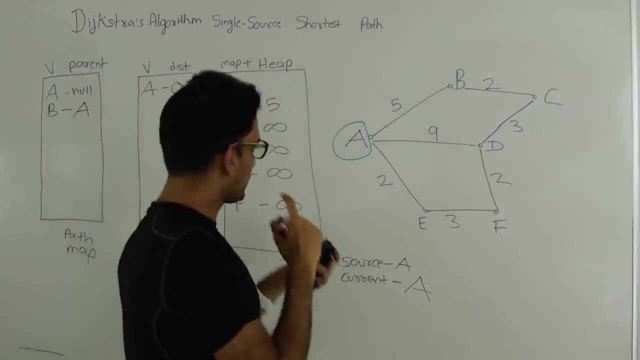 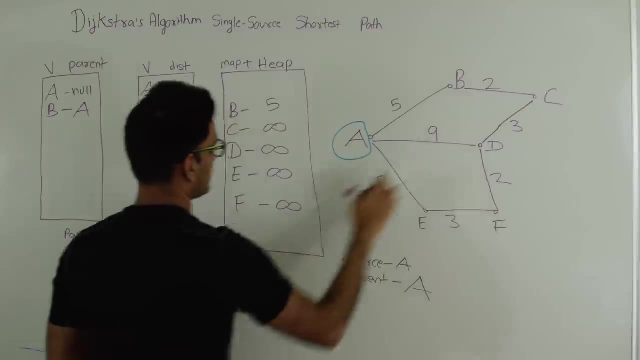 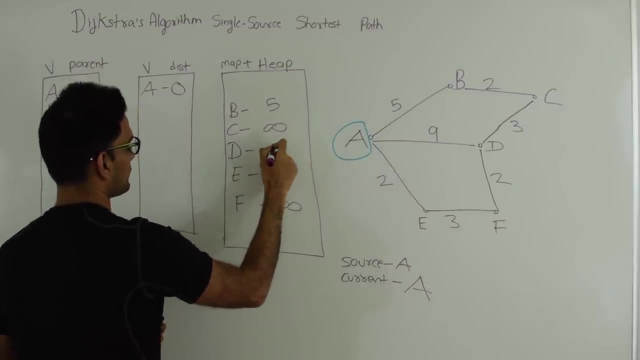 Also. then we're going to explore another neighbor, So D, And then the current distance attached to D is infinity, while this edge, while this guy says that you can reach D from A in distance 9.. So we'll update this with 9 and also say that this 9 is coming from A. 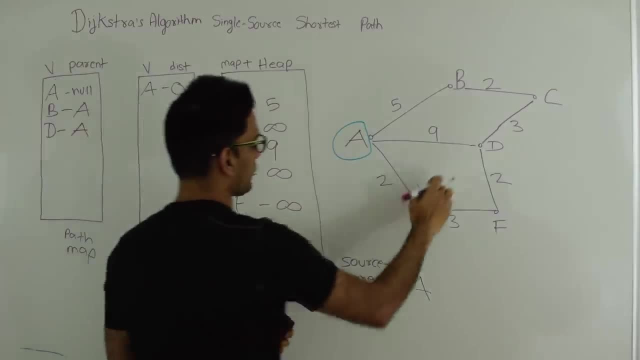 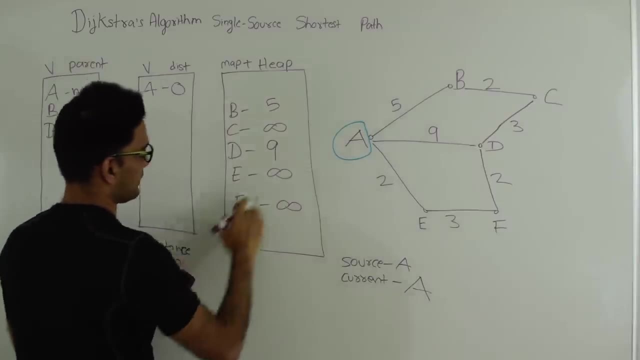 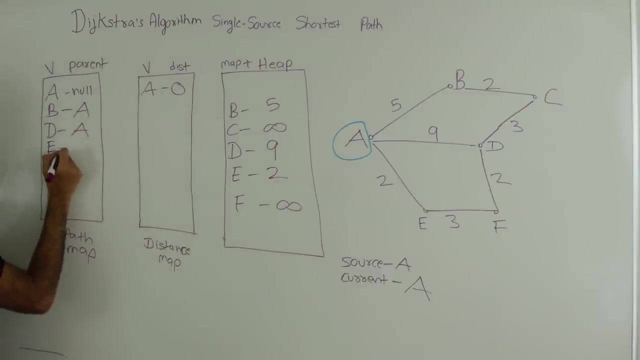 So D is also coming directly from A, And then explore another neighbor, E. So the distance of distance of E from A is 2 and E exists here. so we'll replace this with 2.. And we'll say that E is also coming from A. 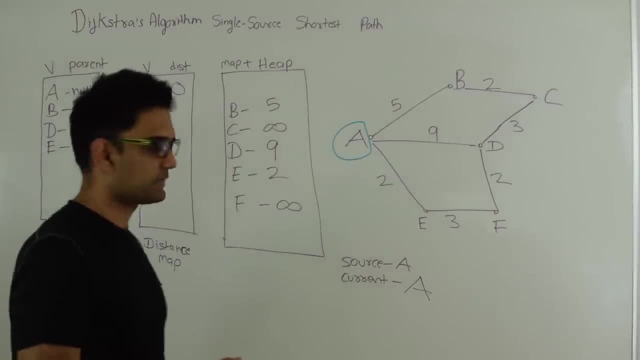 So at this point of time A is totally done exploring all its neighbors. So we're going to go in here again and do another extract mail. So the least value here is E. So we'll take E out. So our current will become E. 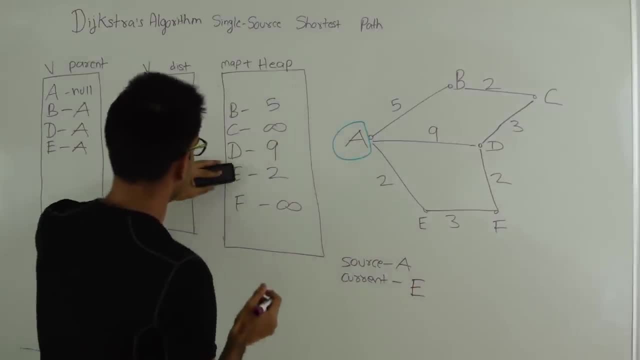 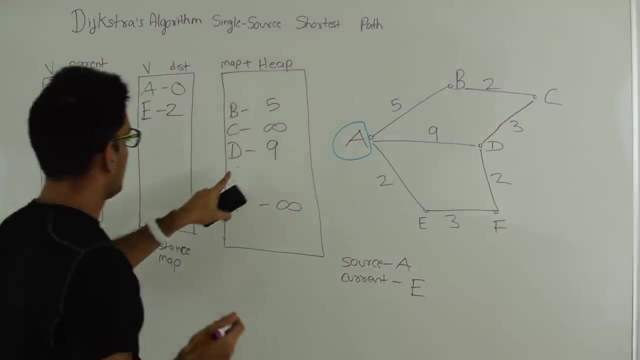 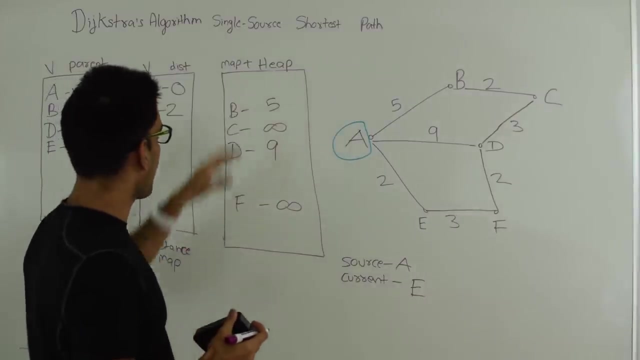 And we'll take E out and put its distance as 2.. And now we'll explore neighbors of E. So the first neighbor of E is A, and A doesn't exist in this map plus heat data structure, so we just ignore A. And then the second neighbor of E is F, and F does exist here. 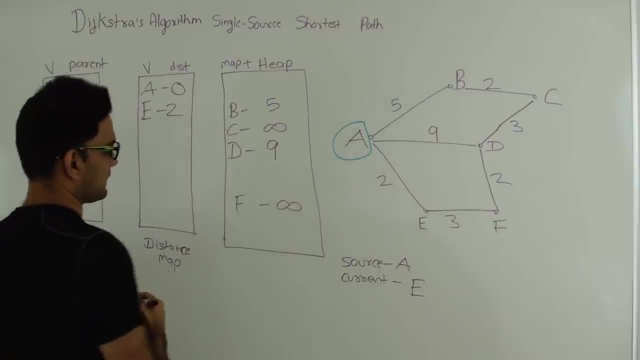 And we just ignore A. And then the second neighbor of E is F, And F does exist here And we just ignore A. And then the second neighbor of E is F, And the value attached with F is infinity, while if we went via E, it can reach A in distance. 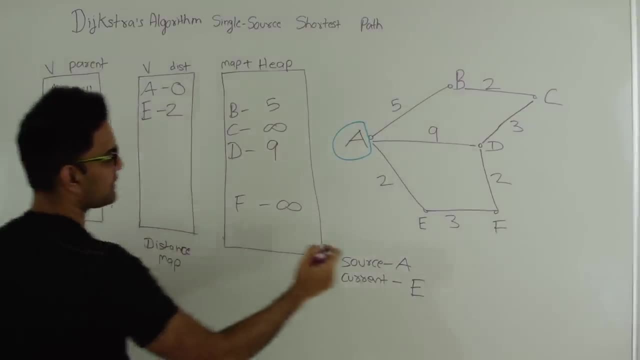 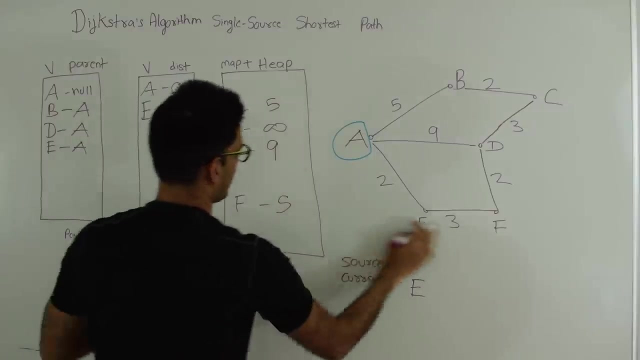 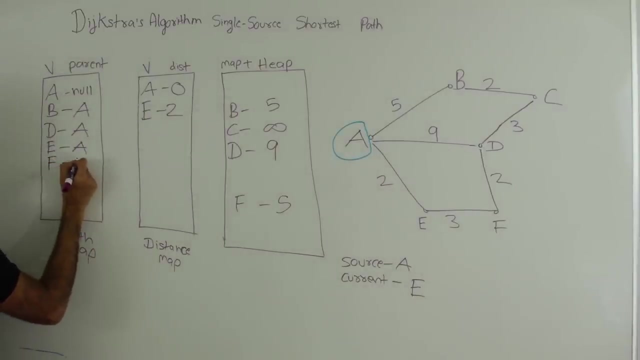 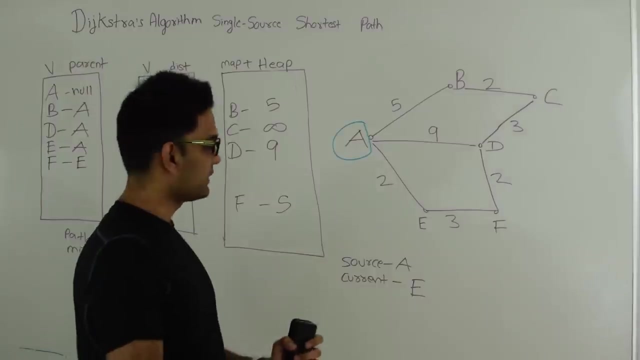 to whatever the minimum it takes to reach E plus the weight of this edge. So value of F goes to 5.. 2 plus 3, 5.. So also we're going to say that F got introduced by E. So at this point of time we're done exploring all the neighbors of E, so we are again going. 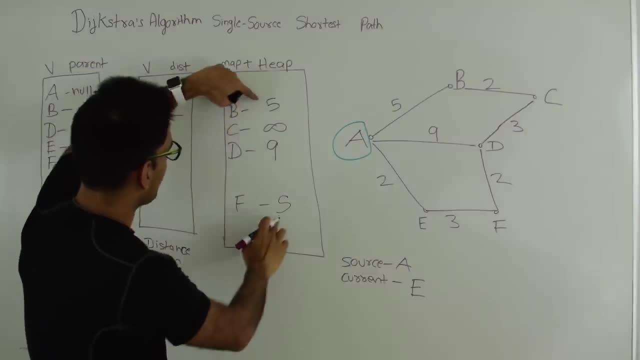 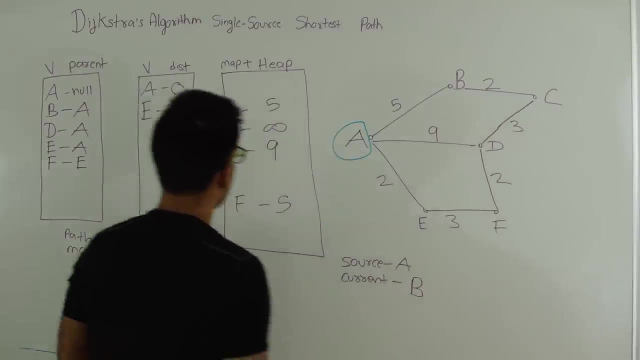 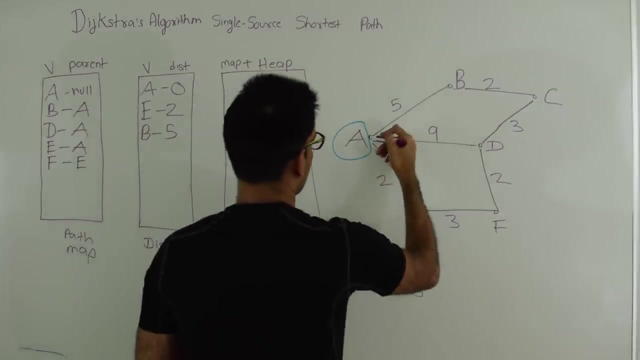 to do an extract min on this data structure so we can pick either of them. So let's pick B And say that the B's minimum distance from A is 5, and ok, so we'll explore neighbors of B. So the first neighbor of B is A, but A doesn't exist here, so we'll just ignore A. 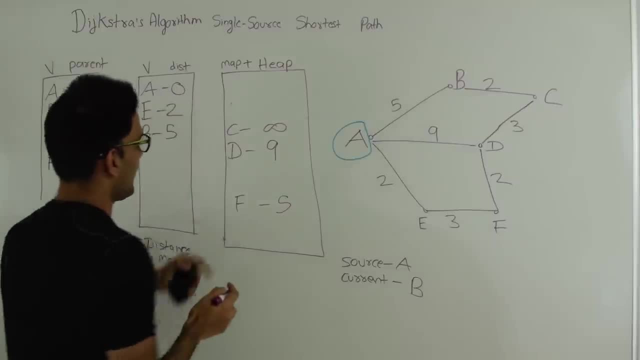 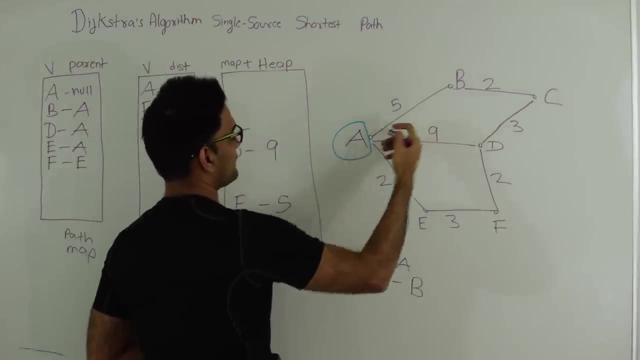 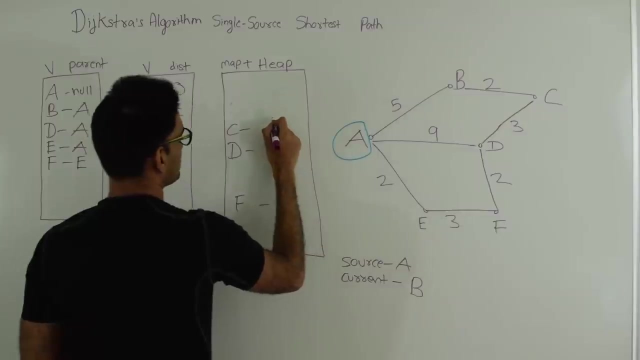 And then another neighbor of A's, B, is C, and C does exist here and the value attached with C is infinity, while if we go via route B, then it can reach A in distance 2 plus whatever is attached with B, so that's 2 plus 5, 7, and then we're going to say that C got introduced. 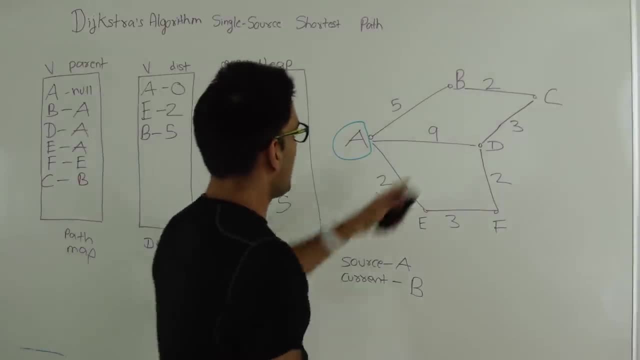 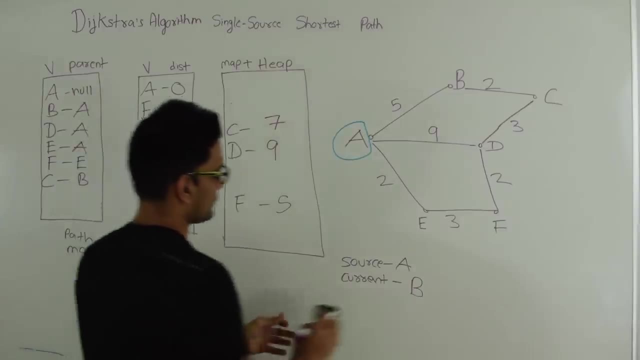 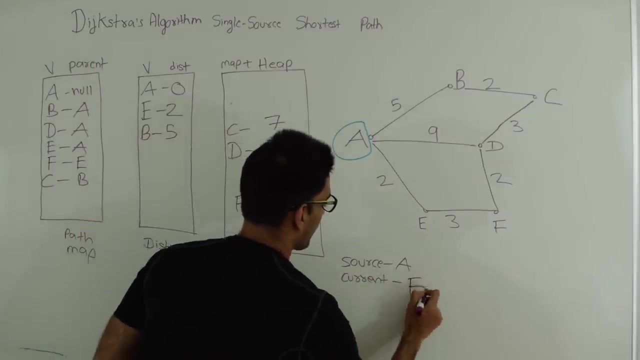 by B, And at this point of time B doesn't have any other neighbors, So we are again going to go in and do an extract min here. So this time 5 comes out, because 5 is the least value of all three. So F is the least value of all three, so F comes out. 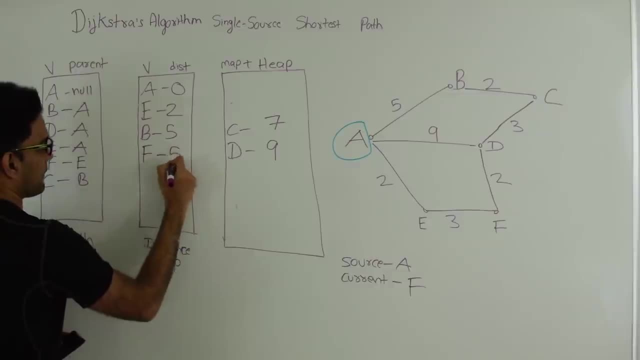 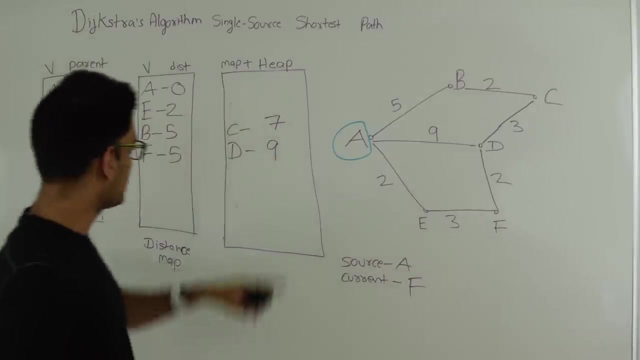 And we're going to update F's distance to 5.. And then we're going to explore neighbors of F. So first neighbor of F is E, But E doesn't exist in this map here, so we're going to ignore E because we've already found. 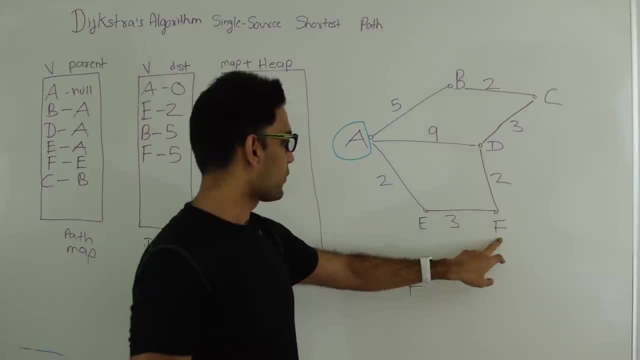 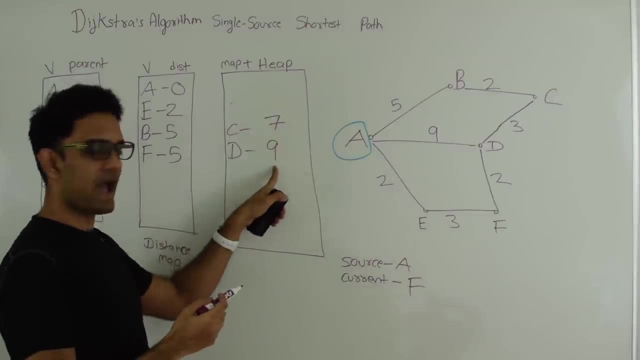 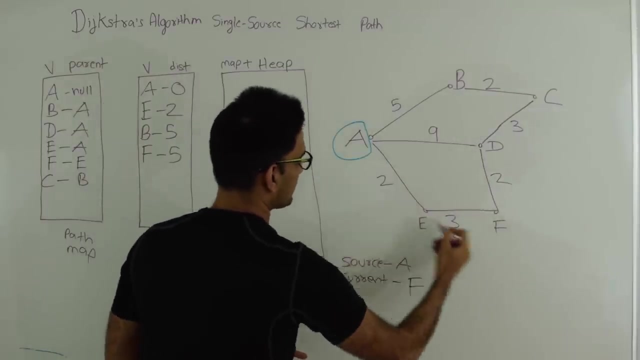 the shortest distance of E from A, Then we're going to explore another neighbor, which is D. So currently D does exist here and currently we found one path to D via this route. but if we took this route, basically this route, we can reach D in a shorter distance, because 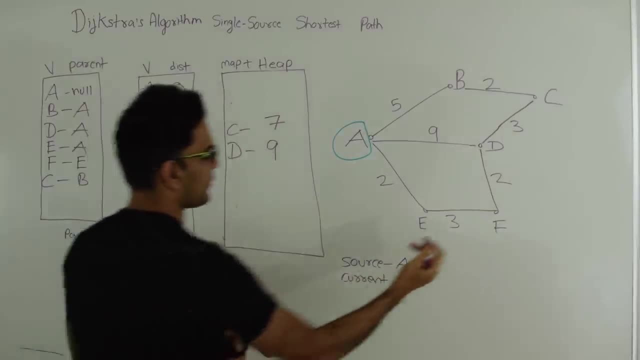 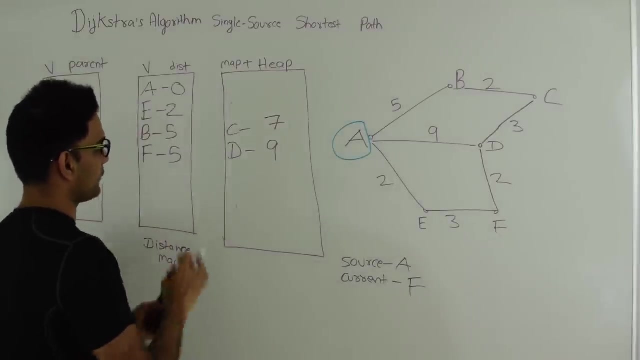 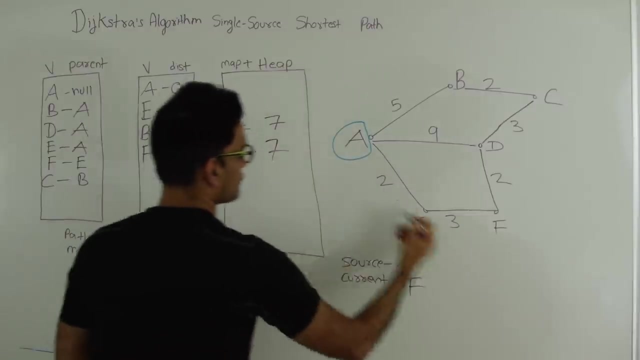 we can reach F in distance 5.. And from F to D it will take 5 plus 2,, 7, so that distance is shorter than what it is right now. so we'll replace D with 7.. So before D could be reached with distance 9. but if we took this path via F and F can 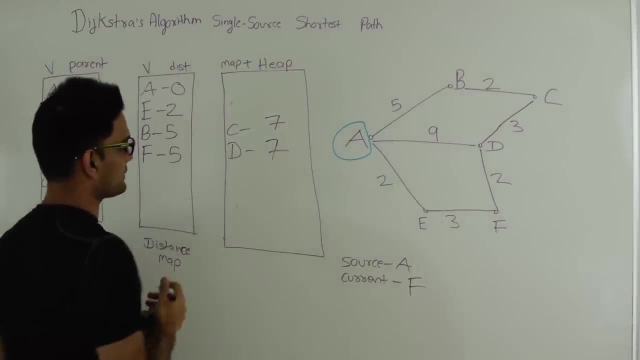 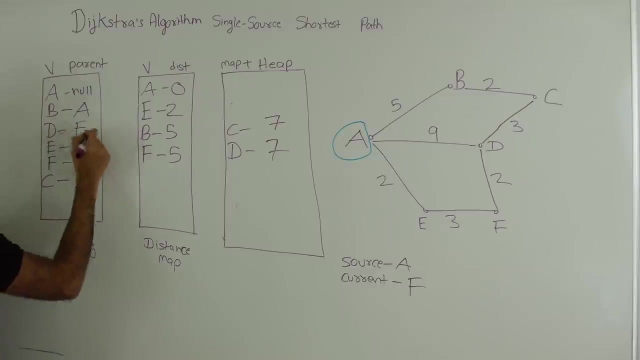 be reached in 5, and the weight of this edge is 2, so we can reach D in 7.. So we're going to go here and say that now D's parent is F, Because that's the. That's the guy who introduced 7 for D. 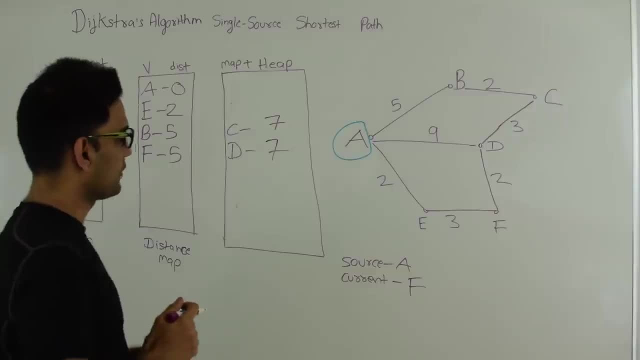 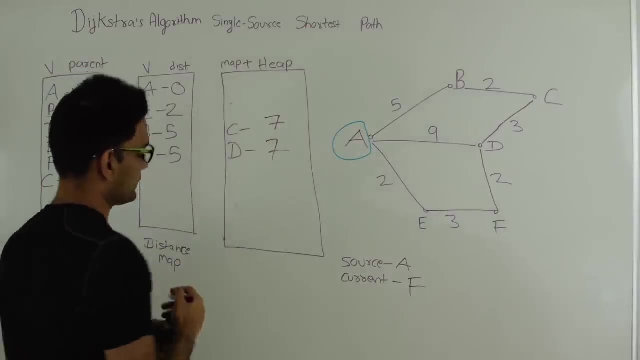 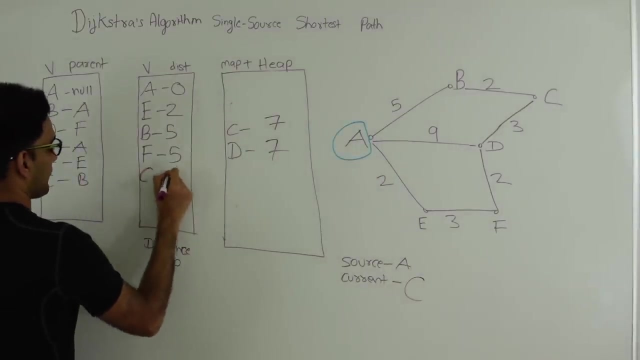 Then now F has no more neighbors to be explored, so we'll go towe'll again, go in and do an extract min here. So let's say we got C out. So our current neighbor is C, Our current value is C, and we'll say C is 7.. 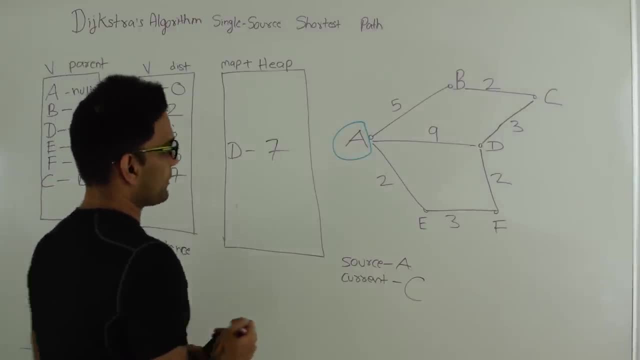 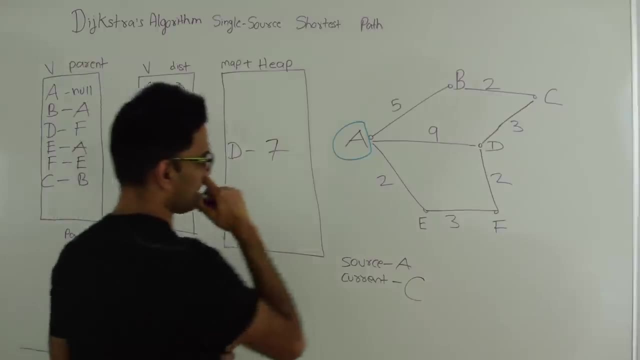 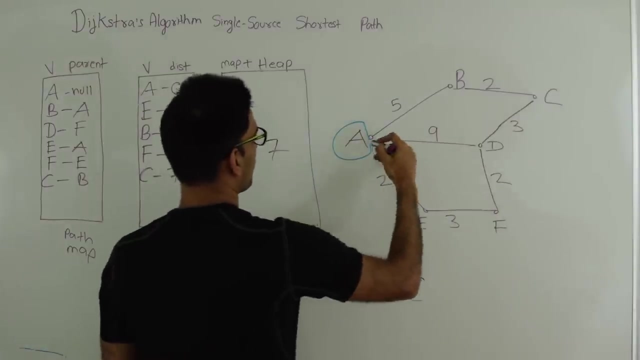 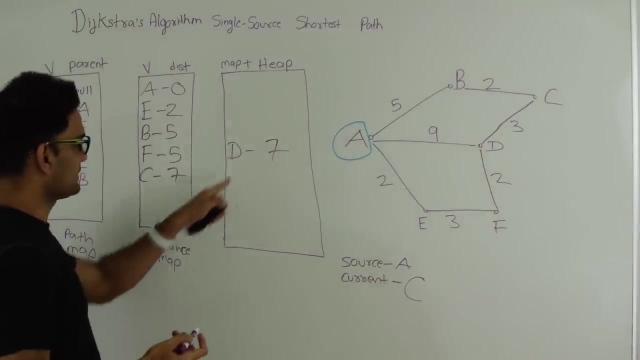 So now we'll explore neighbors of C. So first neighbor of C is B, and B is not here, so we'll ignore B. Another neighbor of C is D, and the value to reach D via C will be whatever it takes to reach C, which is 7, which is 7, plus the weight of this edge, which is 10, which is greater. 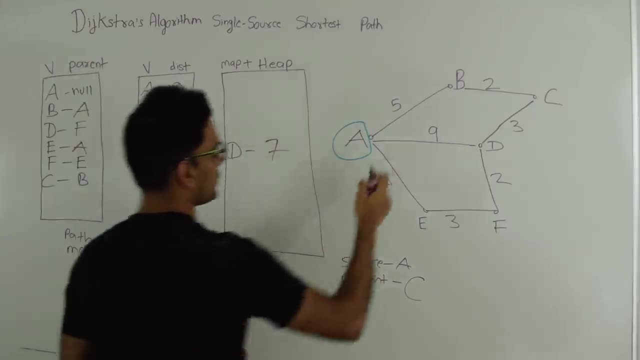 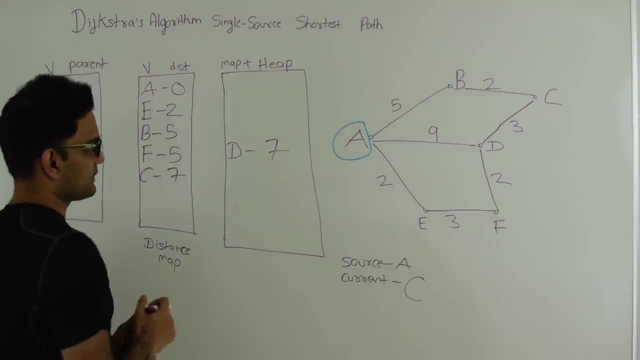 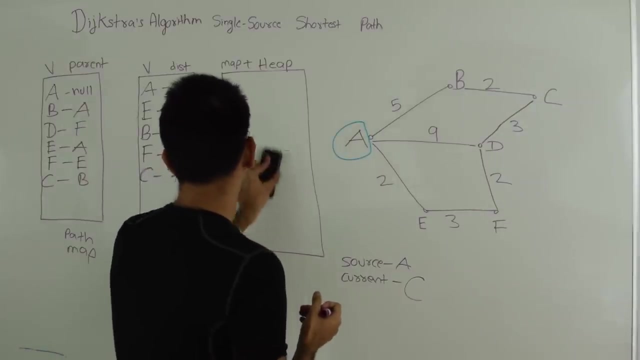 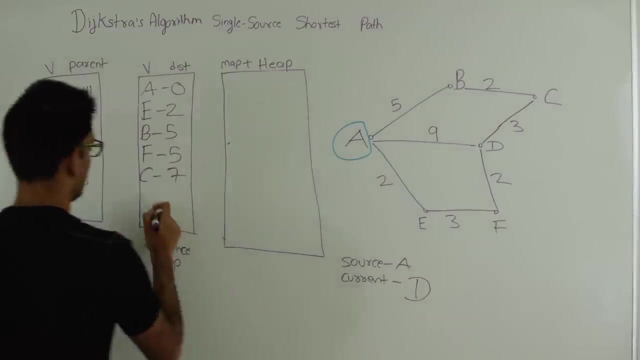 than what we have here. So there is no reason to go to reach D via this, this route. So we'll just ignore that value. So we are done exploring all the neighbors of C. So, finally, we are going to do an extract min here and our current will become D and 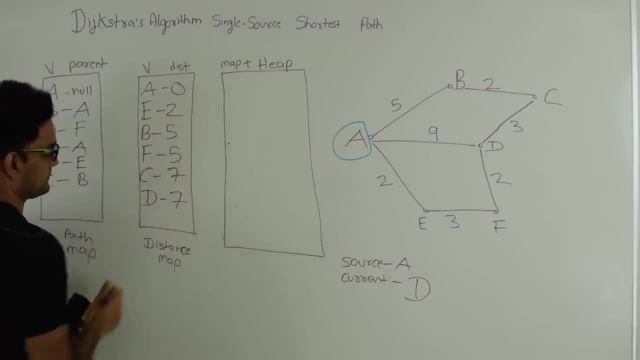 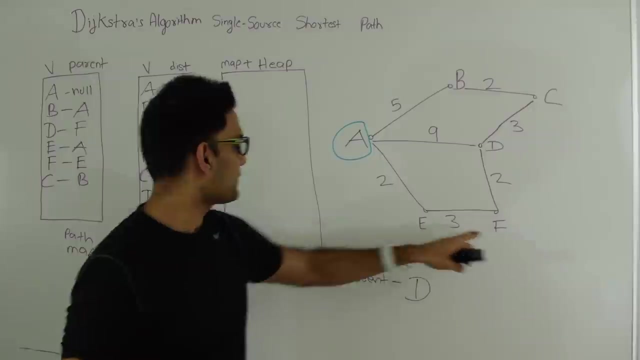 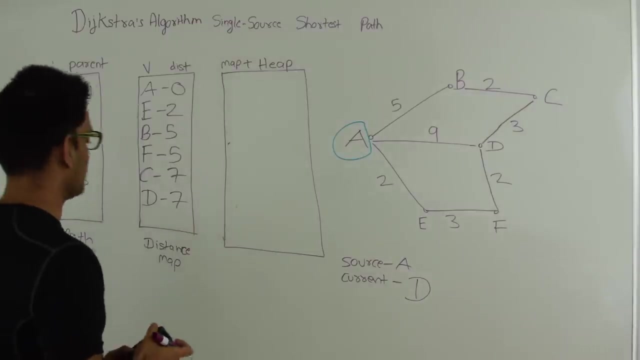 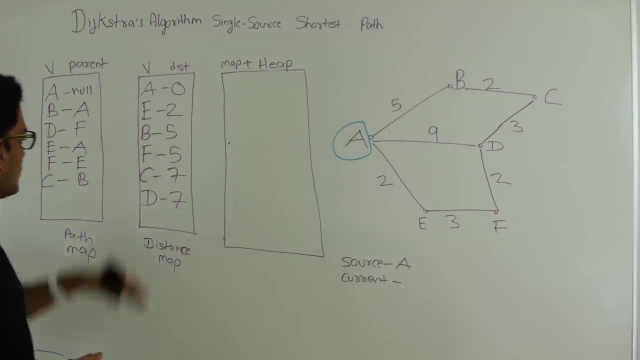 we'll update D, 7, and then D will explore its neighbors: A, which is not there in hereF, which is also not there, And C, which is also not there. So at this point of time we are done with the algorithm. So, because this Qthisthis data structure is now empty, 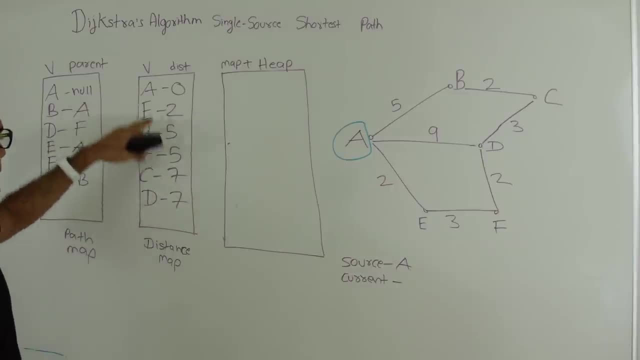 So this is the distance of every vertex from A. E is at distance 2,F is at distance 5,B is at distance 5,C is at distance 7 and D is at distance 7.. If you wanted to find the pathlike howhow to find the pathhow to find the pathhow? 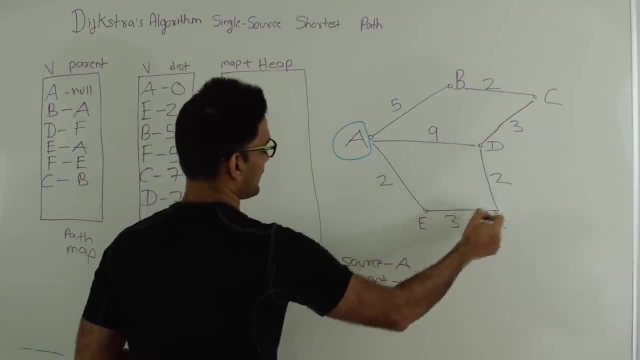 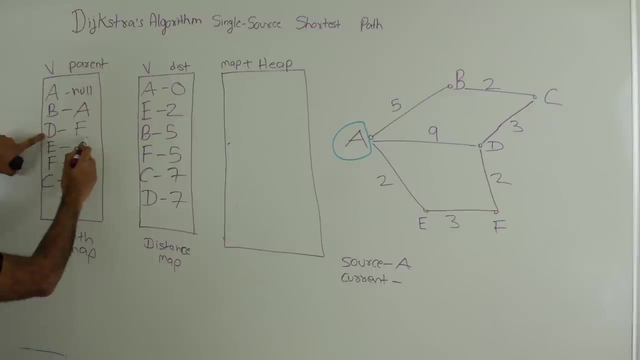 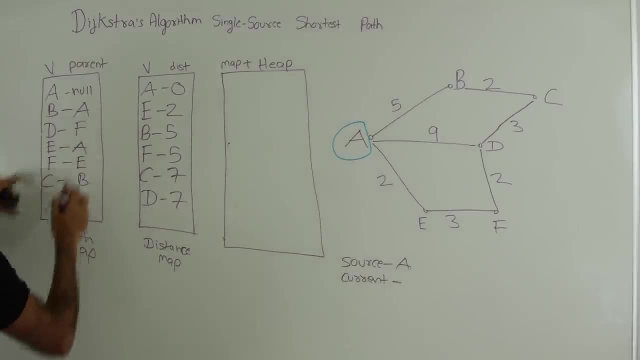 E And then we go to E and E is coming from A, So we can clearly take this path to reach A from D. For another example is: if you want to know how to reach C, so we go hereC is coming from B. 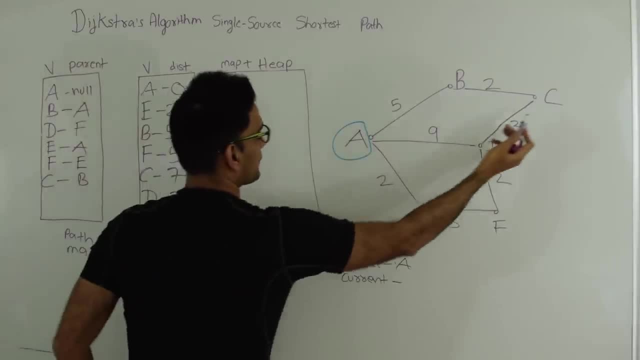 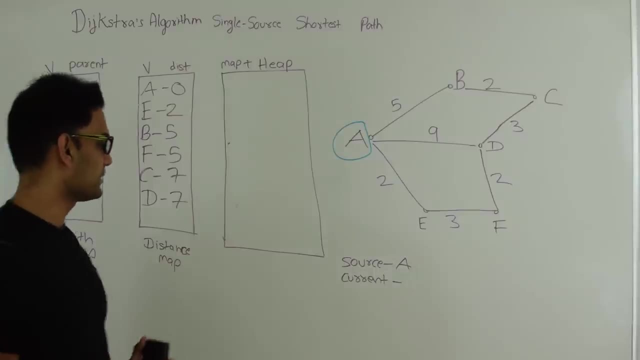 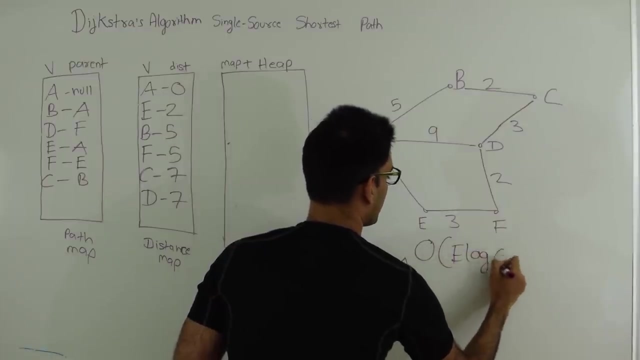 coming from B, and then B is coming from A, so B is coming from A, so we take this path to reach C. So the time complexity for this algorithm is similar to Prem's algorithm, which is E log V. The reason is we are going to apply this. 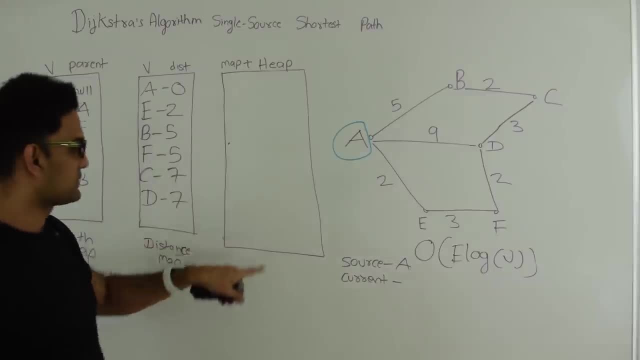 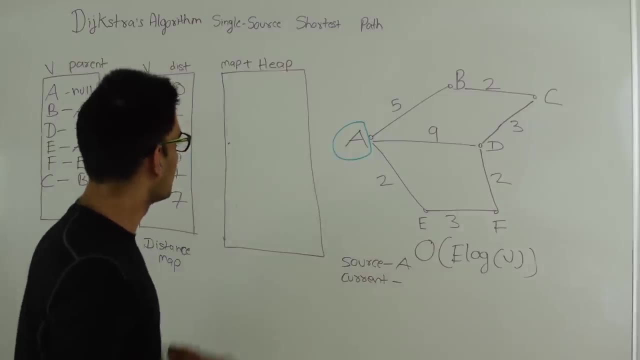 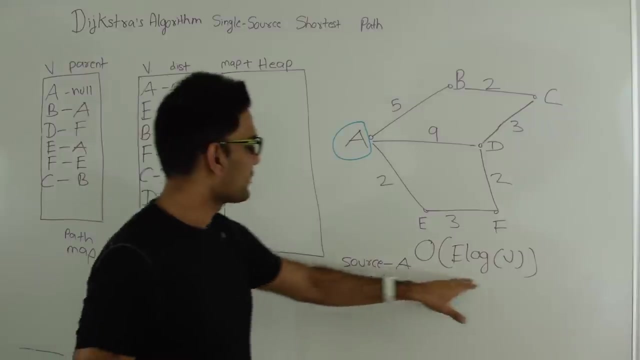 the size of this. this data structure, in the worst case, is going to be V, and then we are going to apply decrease key extract min on this data structure: E times, which is the total number of edges, and V is total number of vertices. So this time complexity will be. 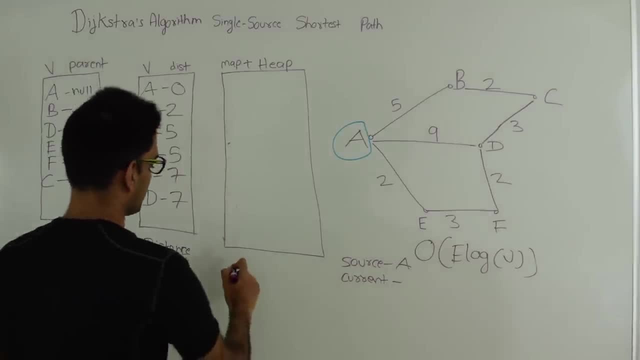 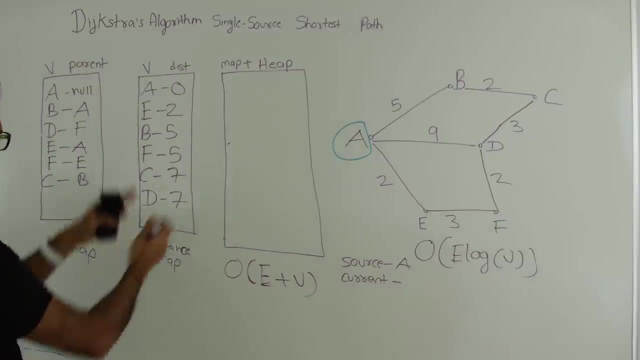 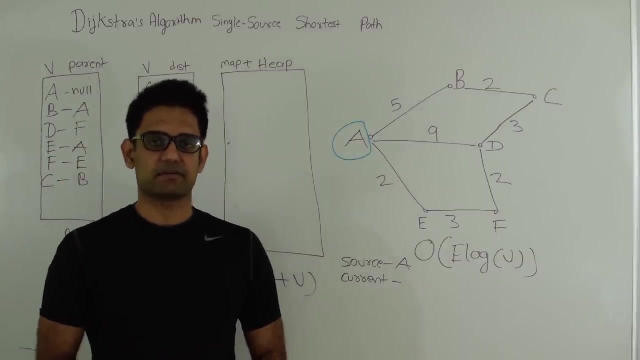 E of log V, and the space complexity will be O of E plus V, because we might have to store as many edges or all the vertices in this three data structure here. So in the next section let's quickly look at the code for this algorithm. 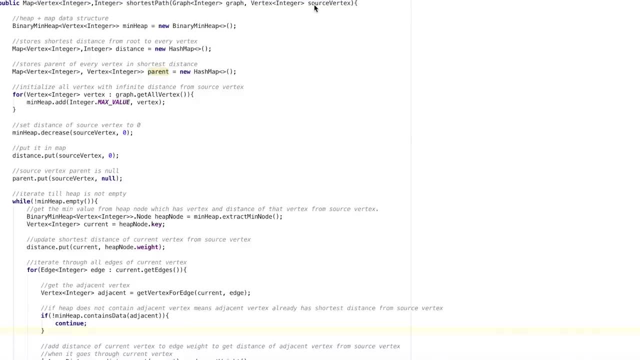 The name of the code is function is shortest path. it takes in the graph and the source vertex from which we want to find the shortest distance of every other vertex, and then it returns a map of vertex and the shortest distance of that vertex from the source vertex. 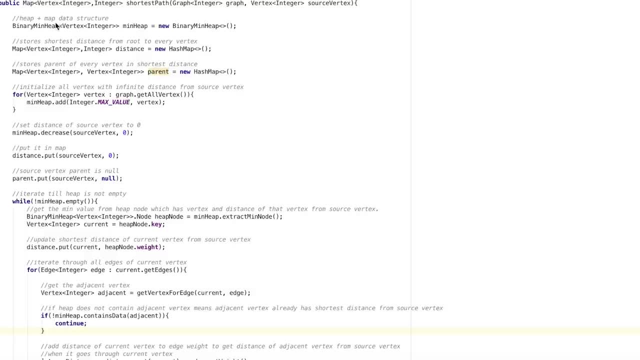 and then let's initialize our data structure. The first one is a heap plus map data structure which supports extract, min, add, decrease and contains operation. and then the second data structure is a map which stores the shortest distance of the source vertex to every vertex. and then this one is a pad and which which is: 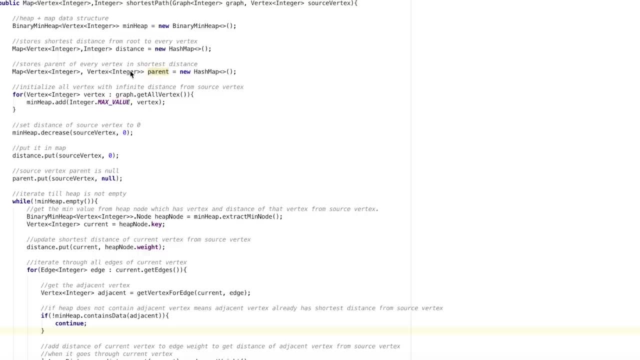 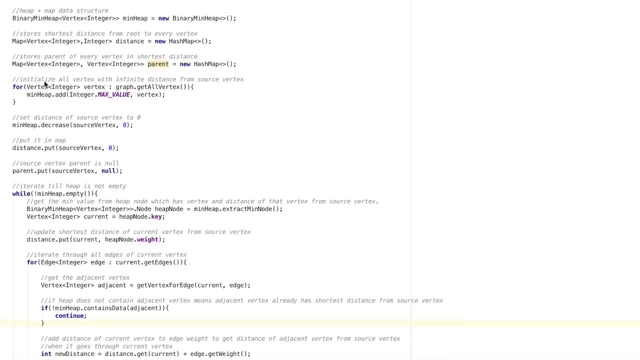 useful for tracing the shortest path from server text to every vortex. The first thing we do is we initialize all the vertices with infinite value, as we discussed before in the video. then we are going to decrease the value of source vertex to zero, because source vertex is a definitions variable, and with that we will be able to circlingентаpe of all vertices and generator and generate system, As we discussed in the previous video. John Stephan has added lead. Don't forget to subscribe. See you soon. 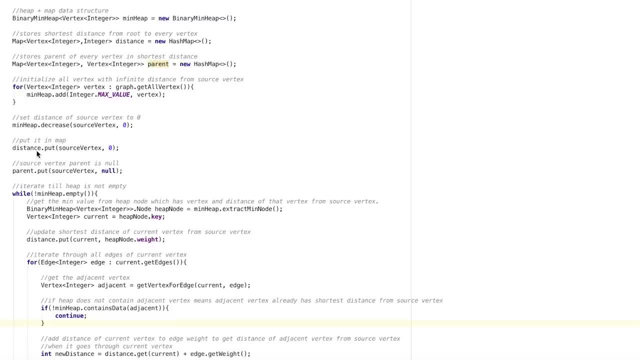 Yac Hazel has added lead from naval facts in delta values to從 concepts. toowu vertex is at the distance 0 from itself, and then put this value in the distance map and also set the parent of the source vertex as null. Now we are going. 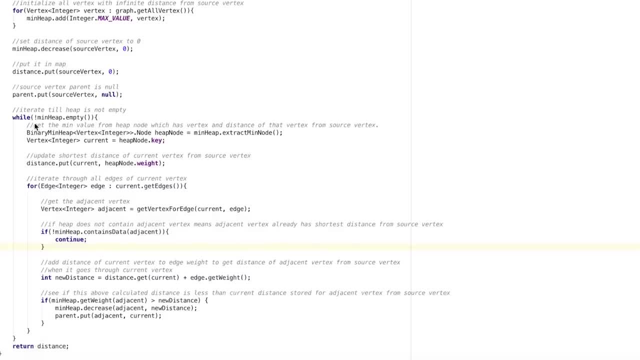 to iterate through the minHip until minHip has elements in it. So then we are going to extract the minimum value vertex from this minHip and it returns me a heap node which has both the actual vertex and the distance of that vertex from the source vertex. Once we get this heap node we get 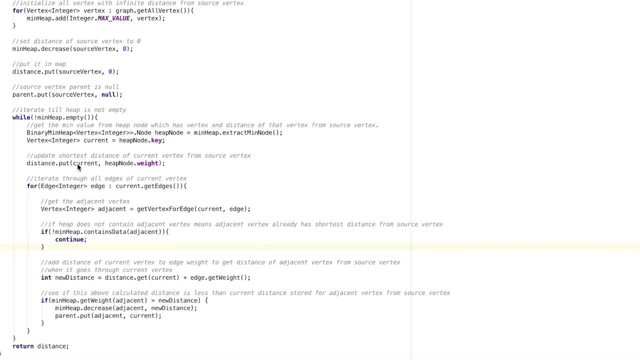 the current vertex from it and also update the distance map. In distance map we put this current vertex and the distance of this vertex from the source vertex. Then we are going to iterate through all its neighbors one by one so we get its adjacent vertex. Then what we're going to check is if the 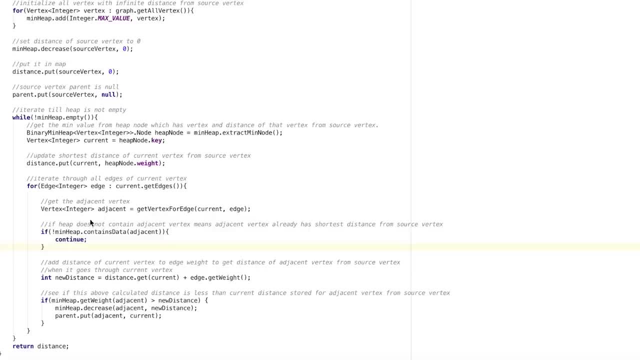 adjacent vertex is present in the minHip or not. If the adjacent vertex is not present in a minHip, it means that we have already found the shortest distance of that adjacent vertex from the source vertex. so there is nothing to do with this for there's nothing to do for this adjacent vertex, so we just continue and go back. 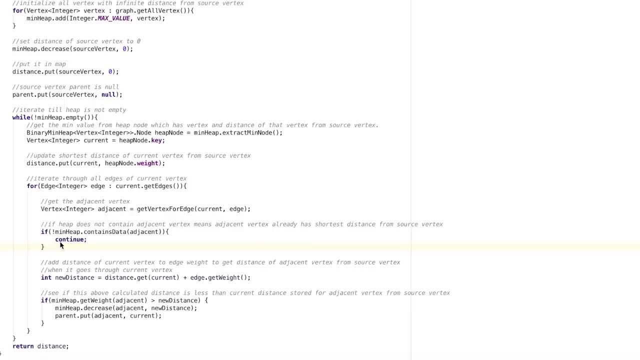 to the top of the for loop and look for the next adjacent vertex, If the minHip does contain the adjacent vertex. so we come to this point and try to find the distance of that adjacent vertex from the source vertex while going through this current vertex. So distanceget current is going to 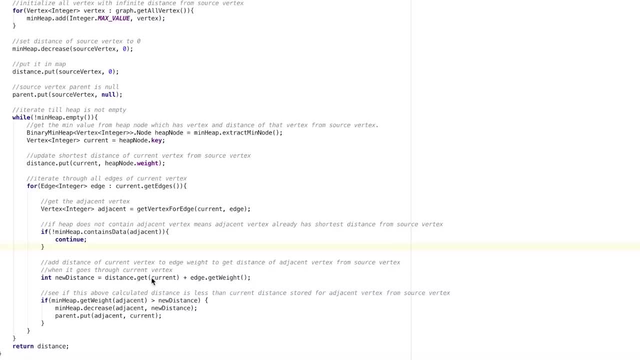 give me the distance, the minimum distance, of the current vertex from the source vertex, and edgegetWait is going to give me the distance between the current vertex and the adjacent vertex. so this new distance is the total distance from a source vertex to the adjacent vertex, going through this current vertex.